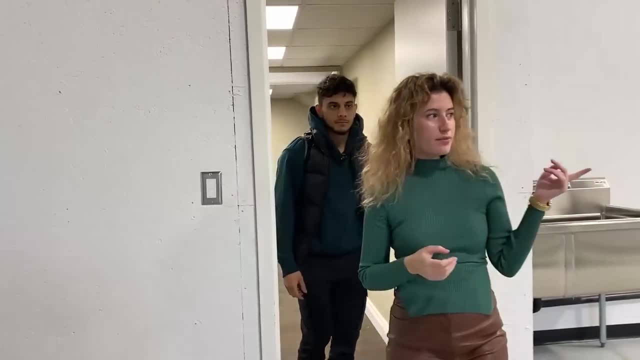 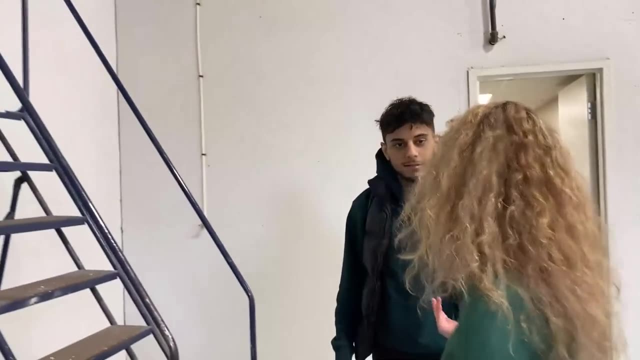 an exit or anything like that. So this is the first lab that we have. This is our new space that we just started working on recently. Yeah, we have a bunch of new equipment. You can spend a lot of time, or you'll spend a lot of time, just doing little experiments and working on stuff. 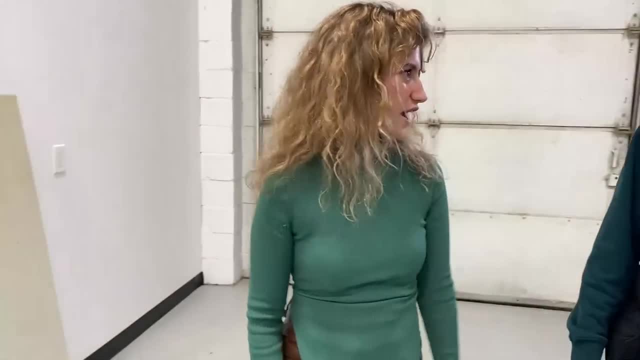 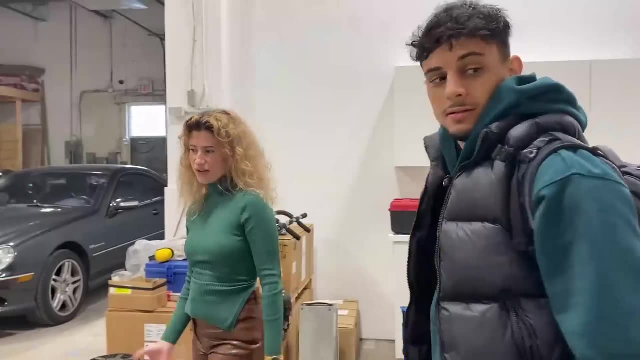 here. But if you have any other questions, please let me know in the comments below, Like: don't be afraid to ask anyone, or to come to me or ask someone and I'll find someone, even if I don't know the answer. Okay, So this is our second lab space, If we ever have like parties. 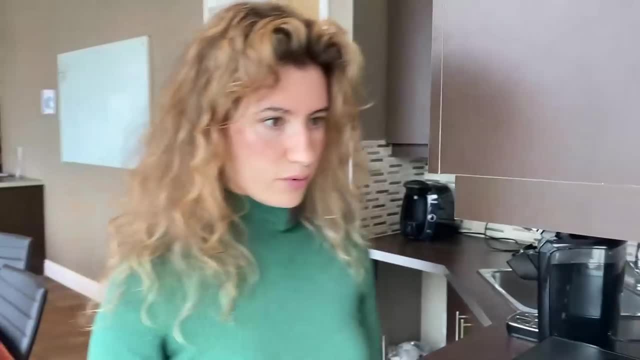 or stuff we can have like a BBQ here, Oh nice. And then this is back where we started. There are some bathrooms right over here. Oh yeah, I'll take you to your desk. Okay cool, This is your. 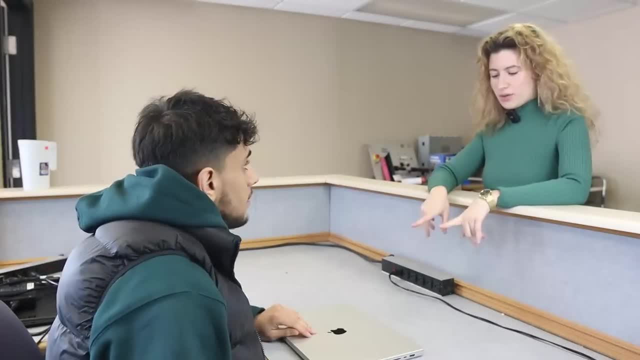 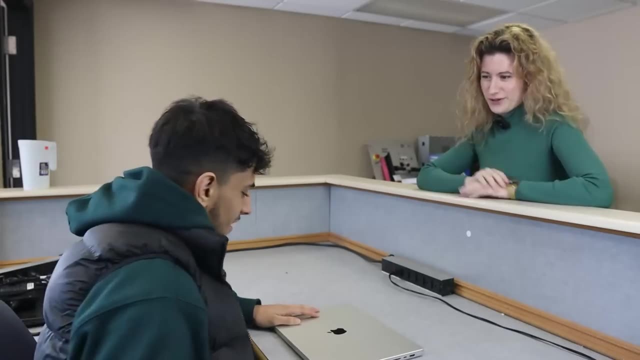 new desk. You'll be working here for the next little bit, And this is your company laptop. Oh, I brought my own personal one. You shouldn't use your personal laptop for work anyway. Oh, okay, Do I need to keep this when the internship ends? No, no. Oh well, it's like a full-time. 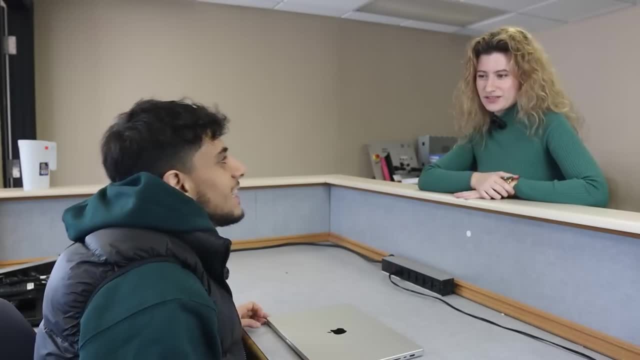 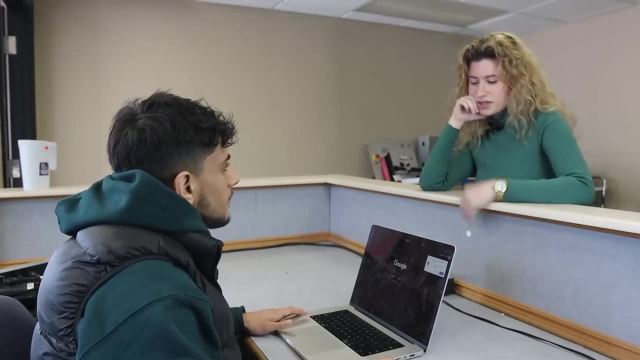 offer. Do I need to keep it? I mean, you could talk to the manager about it, See what they have to say. Okay, You can browse through it and get yourself acquainted with it. The manager should be in about like a half hour- 45 minutes max- and then he'll go over everything with you Besides, 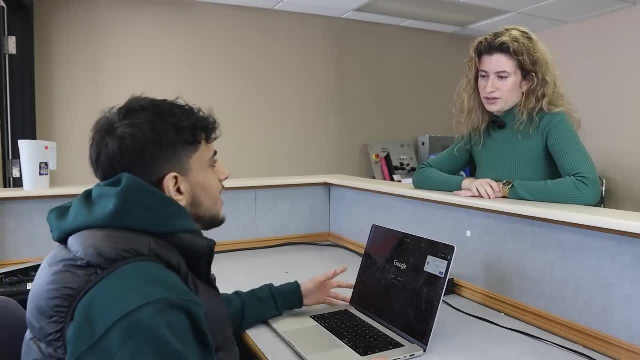 that. do you have any other questions? No, no, I'm good, Thanks. If I have anything, I'll make sure to ask. Okay, cool, Great to meet. you. Have a good day. So excited to finally be applying my. 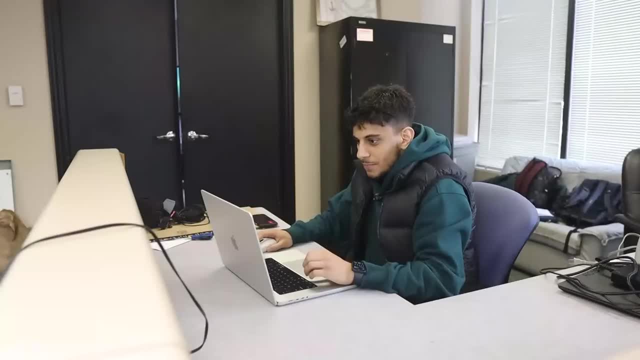 engineering skills in the real world. Enough theoretical stuff. Looking forward to finally starting making some real money now. Hopefully I don't screw this up, You know, even if I do, I'm like just an intern anyways. But you know, no, no, I can't have this. 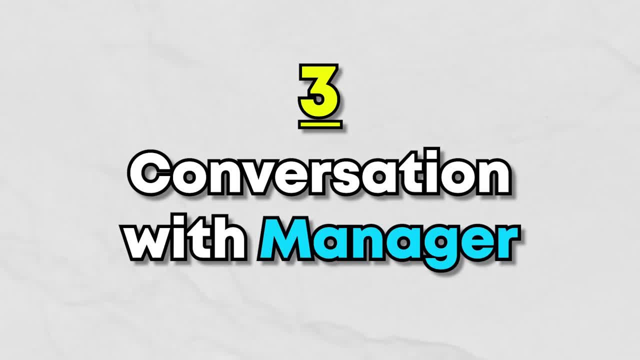 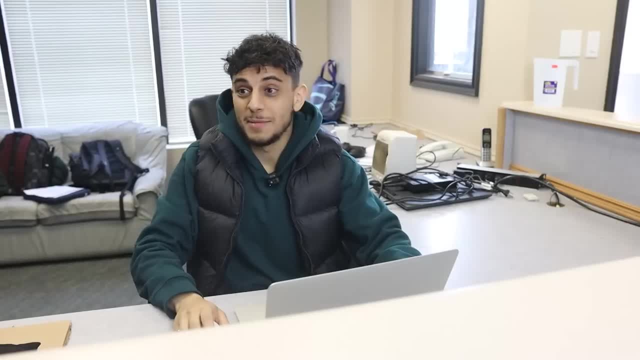 mentality. I'm going to turn this internship into a full-time offer. Hi, Tamer, I'm John. It's nice to finally meet you. You're going to be learning a lot on your co-op term. Yep, I'm excited How. 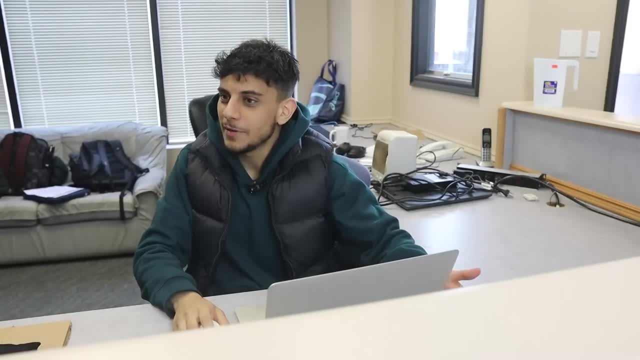 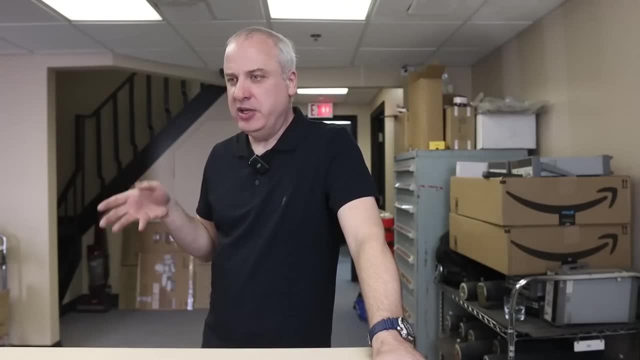 are things going with your laptop? so far, I'm pretty good. I set up my new work email here. so far, I'm just starting to set up Slack as well. Good, There's a few software you need to be comfortable with. Here we use Slack G Suite. 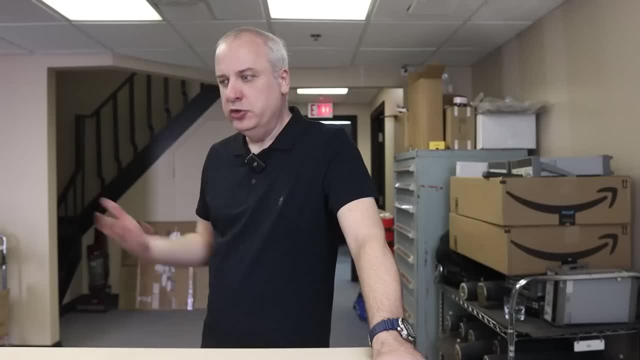 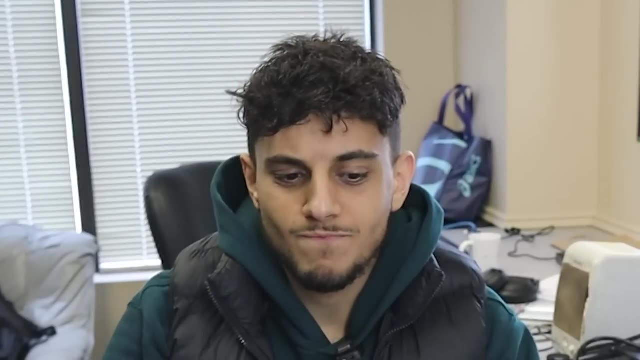 SolidWorks and a few other programs. Oh, what's G Suite, You know, like Google Docs, Google Sheets and Google Slides? Oh, obviously, Come on, Tamer. Why would you ask such a dumb question Now? Slack, most of our communications are on various channels. Make sure you keep your. 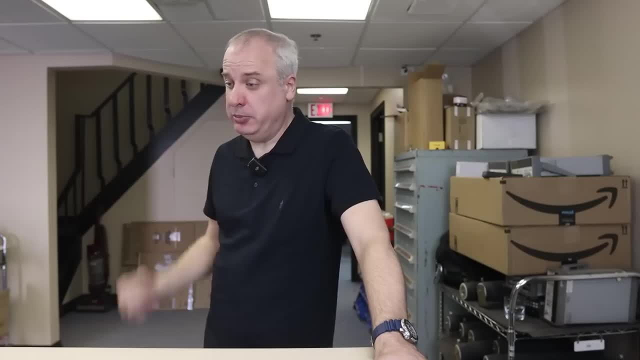 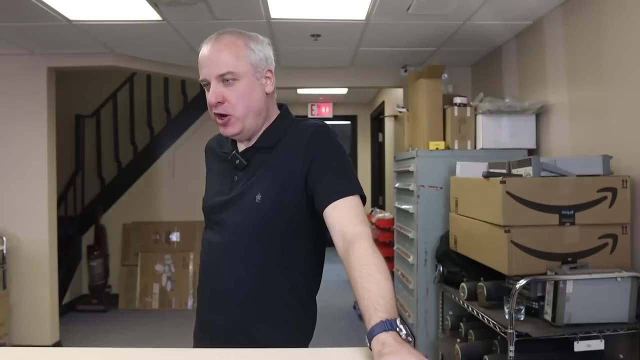 notifications on, because there's more than 50 different places you'll be getting messages from. For sure, I'll set it up right now. Are you ready for your first project, Tamer? Yeah, I just finished setting up my email and installing Slack. Okay, what you want to do next is install SolidWorks, connect it to AutoCAD. 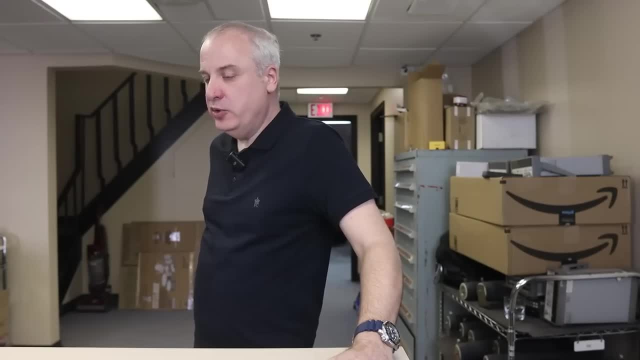 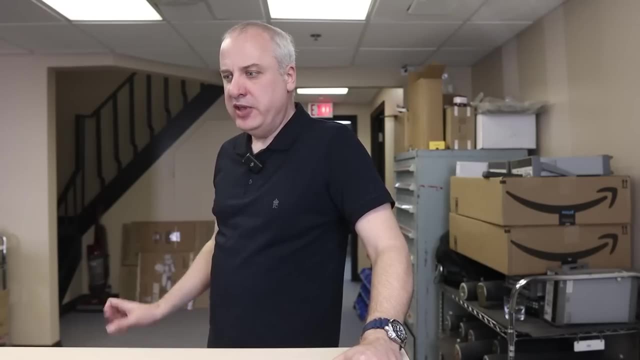 log in with your email to see all of your different files, then use Jira and a few other applications in order to make sure you know how the project's going. Once you're done with that, we must keep track of our bill of materials. We do that using Arena Solutions. You'll definitely 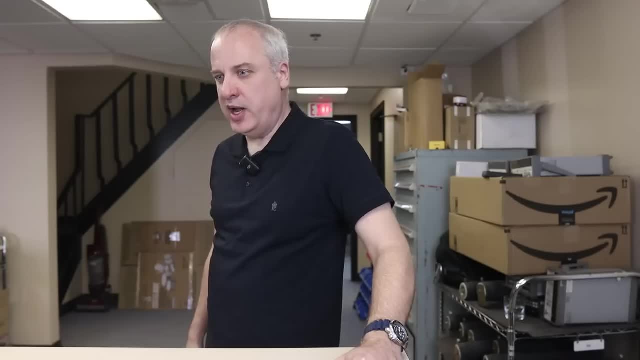 be creating a ton of change orders and change requests, so it's super important you keep organized and up-to-date. Do you have any questions? Yeah, I'm going to go ahead and set up my email and install Slack. I'm going to go ahead and install. 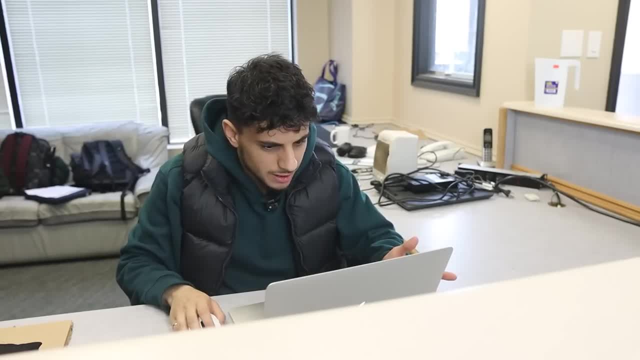 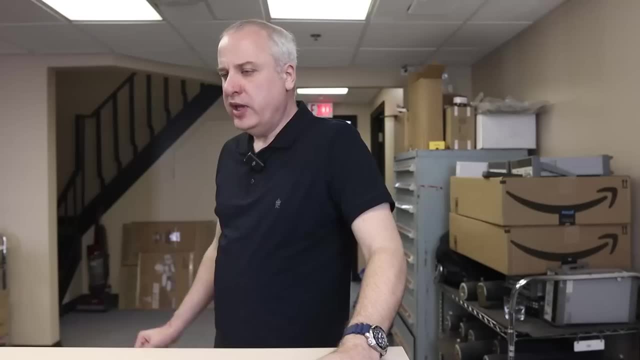 SolidWorks. I can't really seem to find the download button on SolidWorks' website. Oh, do you have access to our Jira G Suite mainframe? SolidWorks should automatically download. once you have access to it, Okay, email our IT team and they should give you. 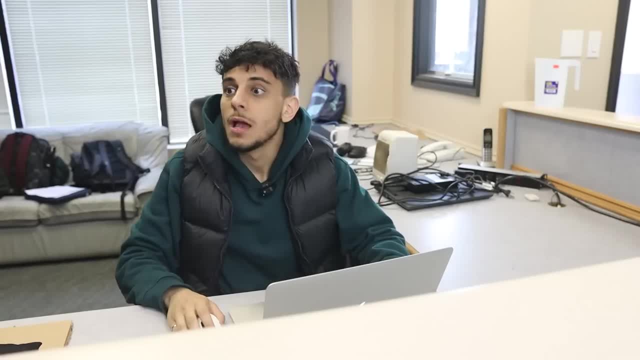 access pretty quick. I have to jump into another meeting right now, so I'll let you figure it out. Oh, okay, Makes sense. Okay, before I forget, can you come to my office in 15 minutes? I got a bunch. 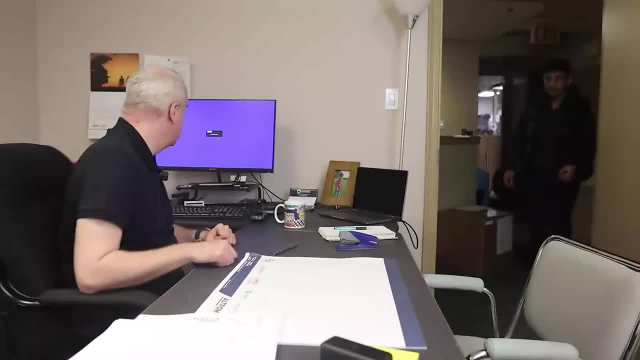 of forms for you to sign. You wanted to see me- Yeah, come on in. So I got some paperwork for you to fill out. I'm going to go ahead and set up my email and install Slack. I'm going to go ahead and. 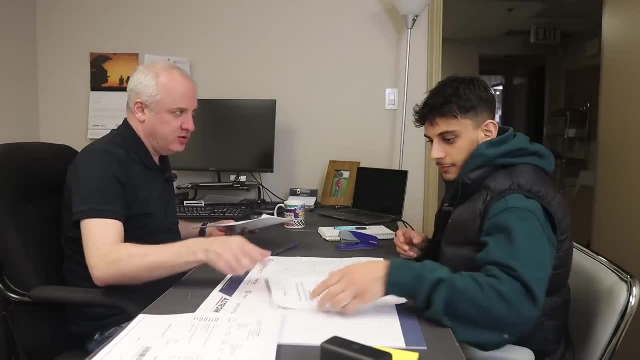 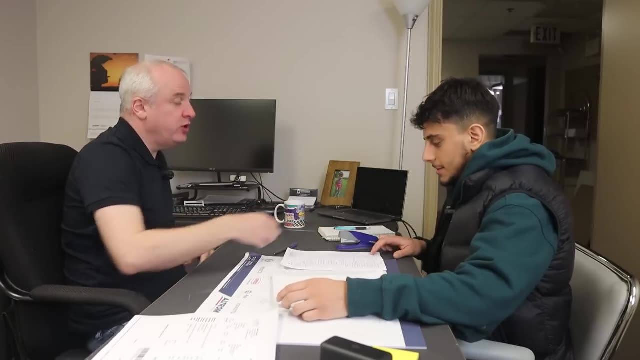 Okay. So, first of all, we'd like you to fill in this: This is your non-disclosure agreement with the company. Okay, Secondly, for payroll, I need you to fill in this so you get paid the end of the month like everyone else. Okay, cool. And finally, I need you to fill in this: That's your 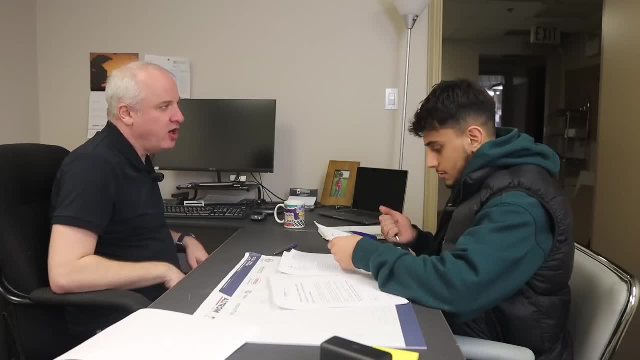 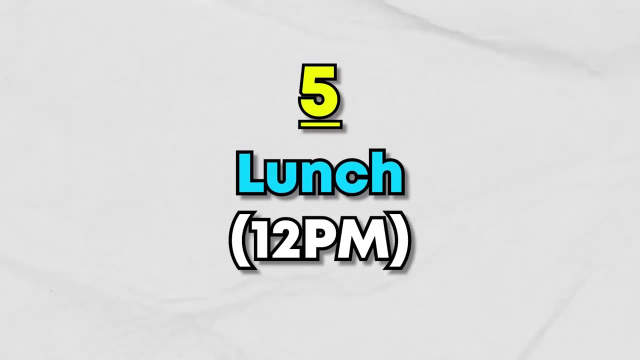 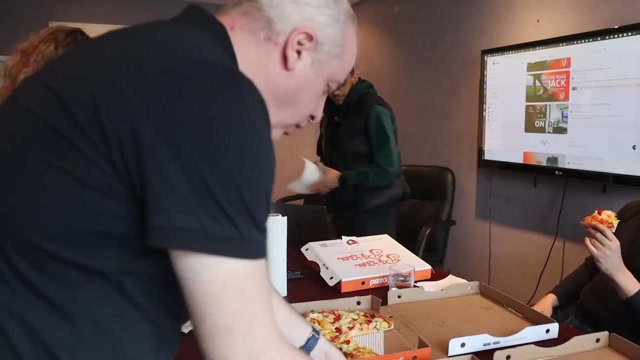 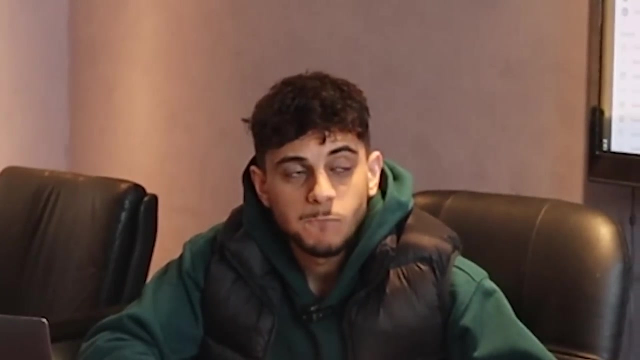 emergency contact form. That way, if something goes wrong, we can contact your family. Okay, sounds good, Thank you. Thank you, This pizza's pretty good Man, but these guys are just talking about their other coworker. Maybe I'll. 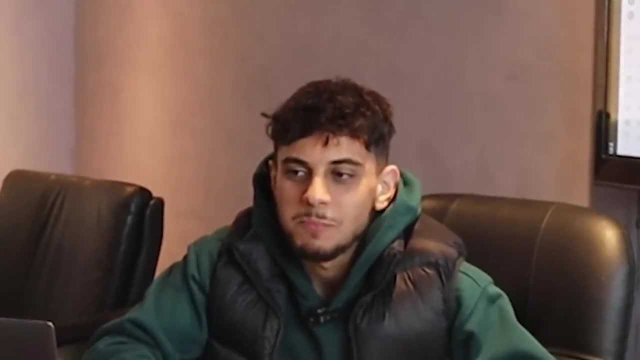 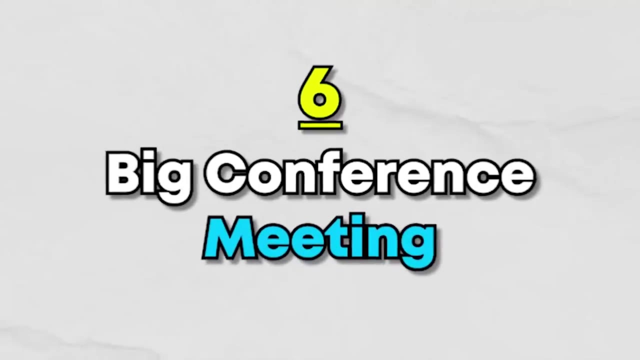 just pretend like I know what they're saying. Okay, that makes sense. Yeah, I'll just keep nodding and smiling. Hopefully they think I know what they're talking about: Amplitude modulated radio. So if you wanted to make a receiver for AM radio, you'd build a peak. 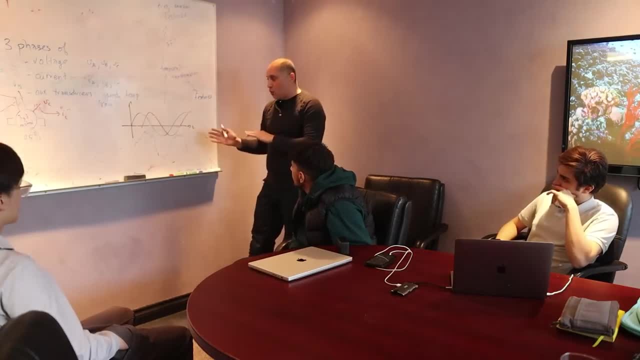 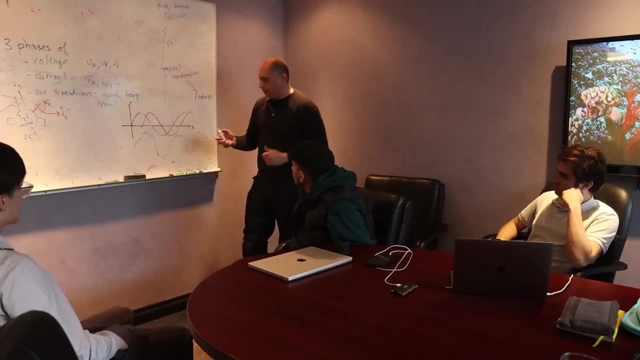 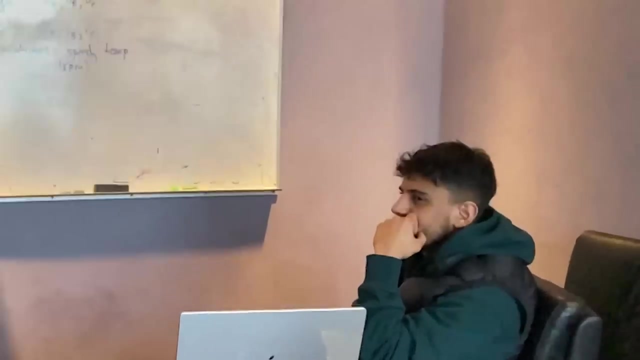 detector. So we just get the broad features and maybe the zero crossings. How many meetings do these guys have? I was exhausted after just one, So we can measure speed. So when you do the envelope detection, do you guys have a favorite algorithm for that? We apply three. When does my 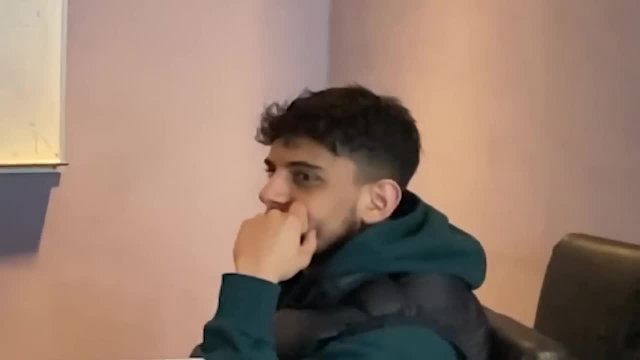 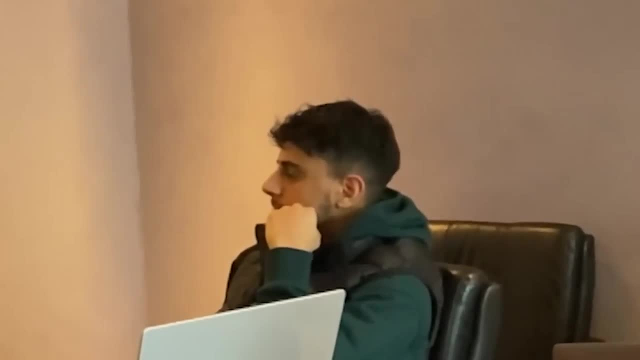 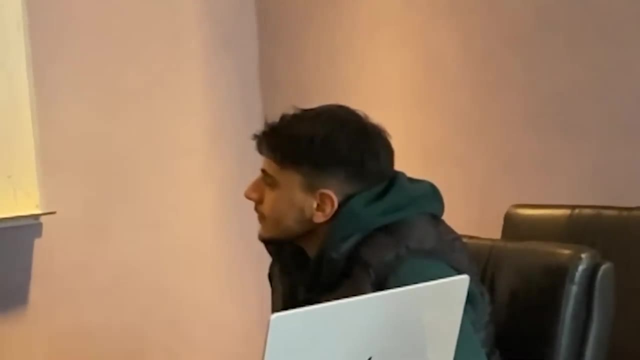 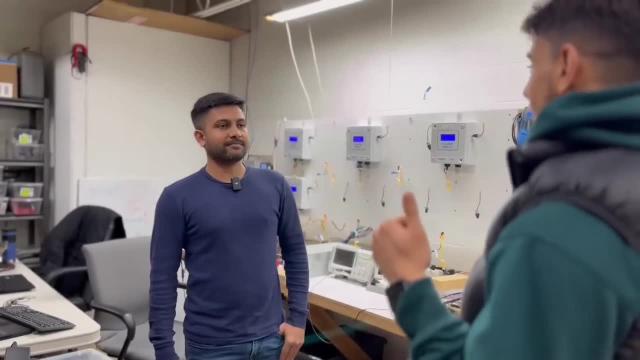 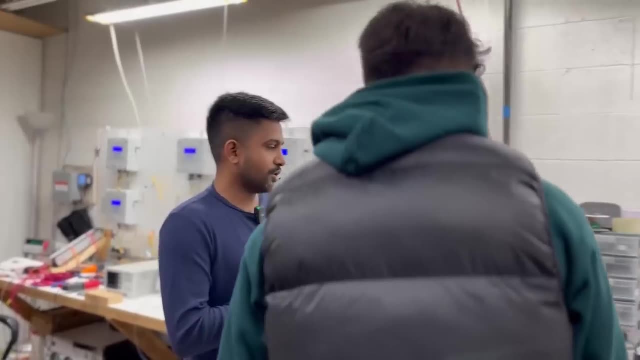 Ankit. Hey, my name is Ankit, So John told me to come and talk to you. I'm the new mechanical engineering intern. Okay, You told me just, you know, get to know a little bit about the electronic side of the product. okay, yeah, so here, like mostly, we do the research stuff. 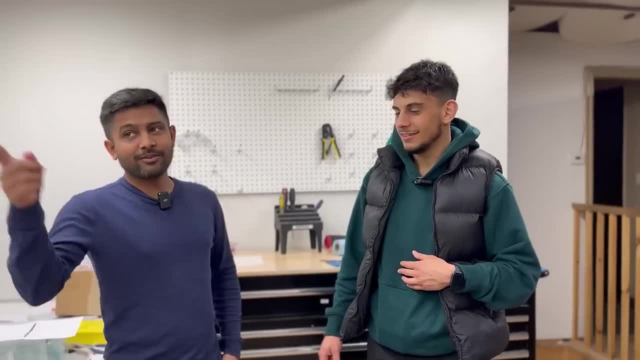 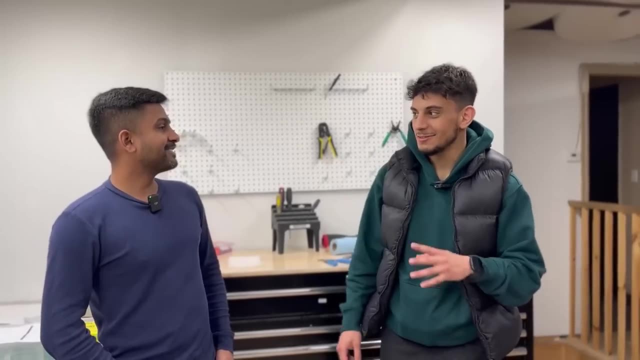 okay, and new development? yeah, no, what's edge computing? that's what we are doing here. edge computing- wait what? this is kind of going over my head. oh, i've like on the electronics. i don't know much about edge computing. what is edge computing? edge computing is you have like, okay, you. 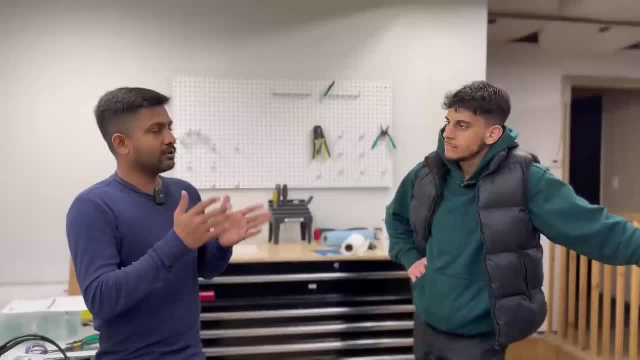 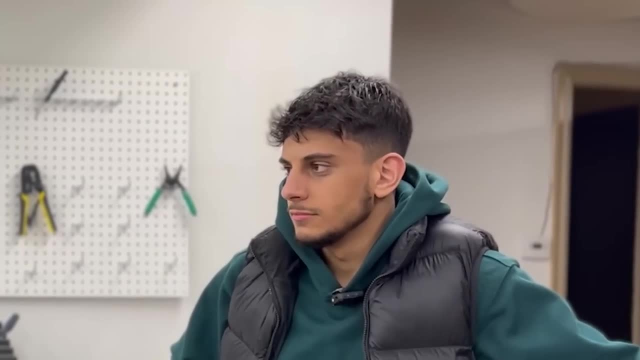 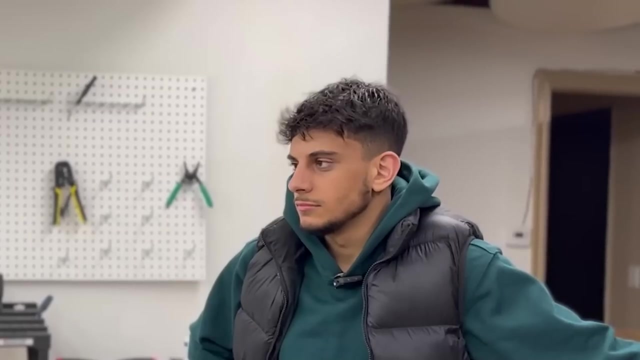 know what tamer focus. just try to understand what he's saying. isolate physical world from the real, let's say cloud or software world. the real world and software world- okay, got it. so in our case, our device is like doing edge computing in means. oh, here we go with this edge computing thing. i. 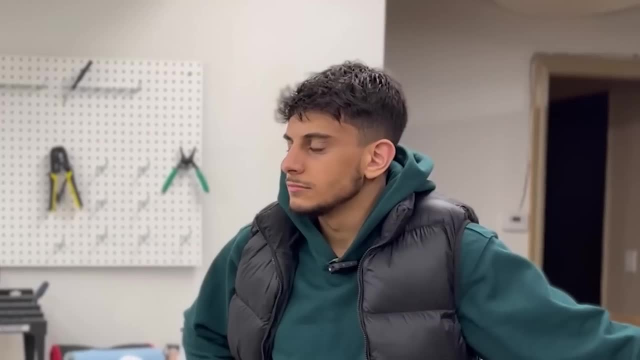 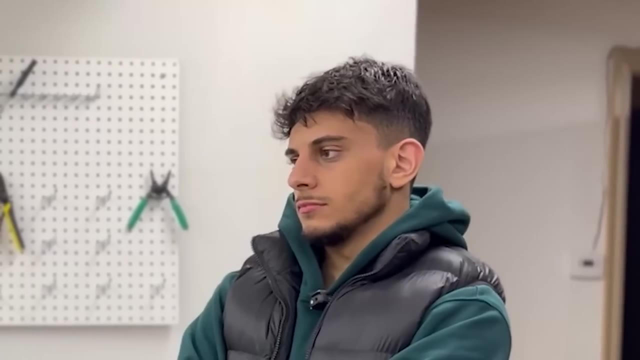 don't remember ever learning this in class. my prof was just teaching me how to take triple intervals and handle efficiently. that is what edge computing okay. okay, let me just ask him a question, so you know i can seem smart. did you learn that in school or just learn it here at work? 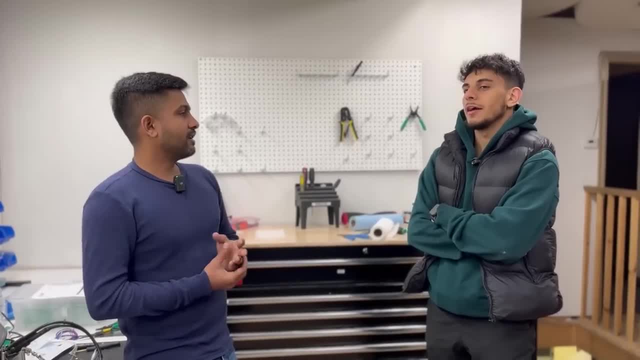 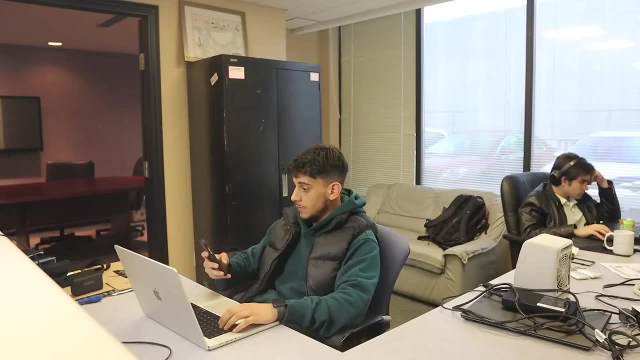 like part of the electronics. oh yeah, he definitely thinks i know what i'm talking about. okay, time for me to head out, or wait. would it look bad if i leave this early? should i just sit here a little longer? uh, okay, my manager is still in his meeting, so i'm gonna just leave. 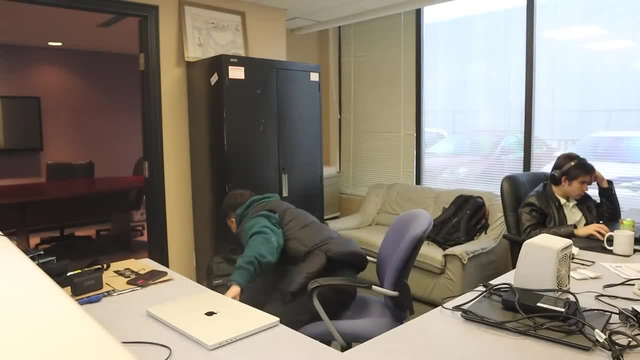 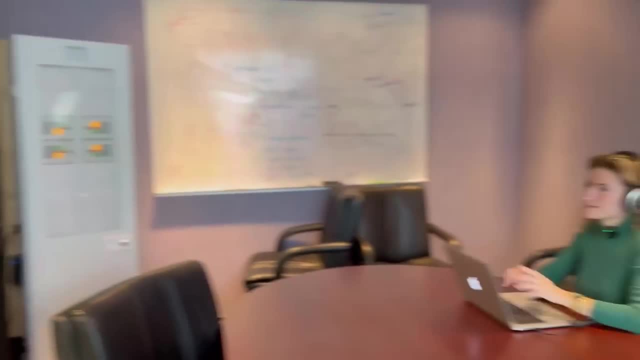 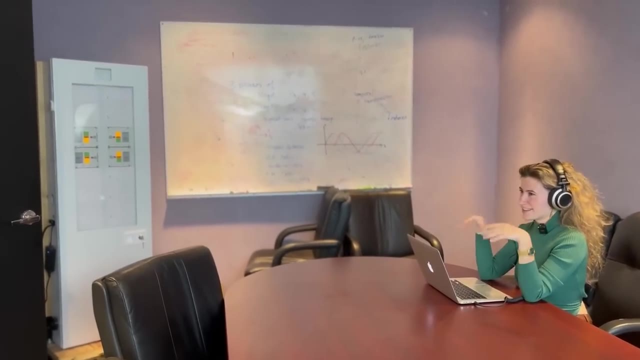 yeah, i'm gonna just head out. it's been a long day, hi, what's up? hi, i'm just gonna head out. do i give this laptop back or no? no, you can take it home and then give it back at the end of your term. okay, i'll get full time, don't worry. yeah, yeah, for sure, 100%. 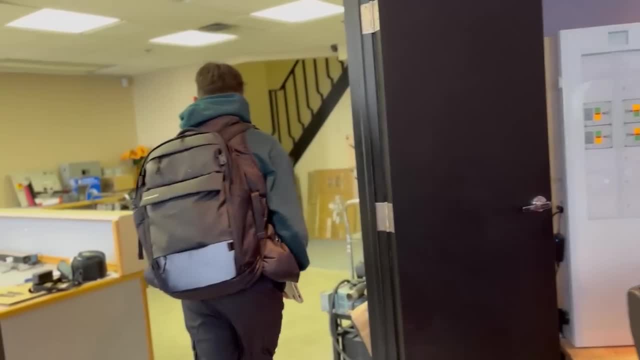 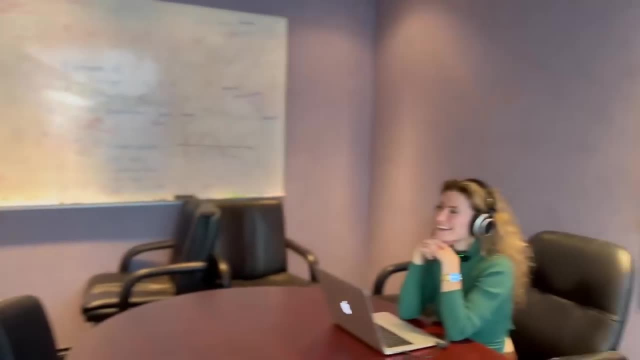 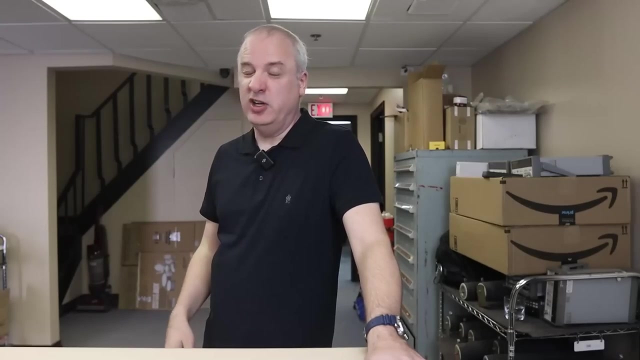 all right. uh, i'll see you tomorrow, yeah for sure. all right, fine, all right, let me just stop laughing. hi, well panned to her. yeah, you're gonna be learning a lot on your co-op term. you're not a co-op though, are you? this is our office space. we have some offices here. we have some workspace here. 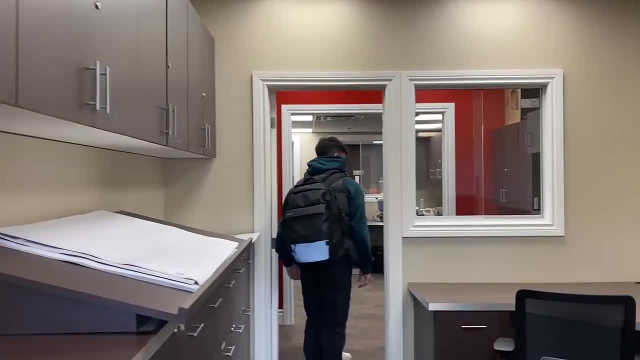 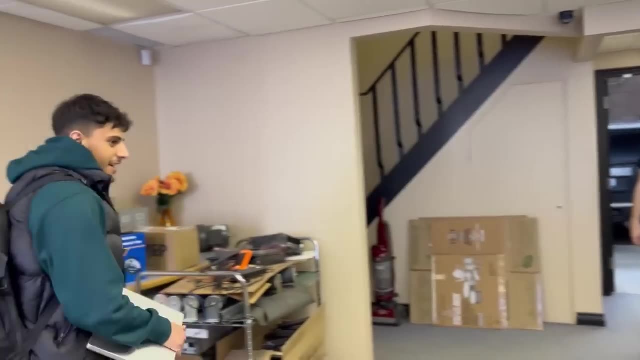 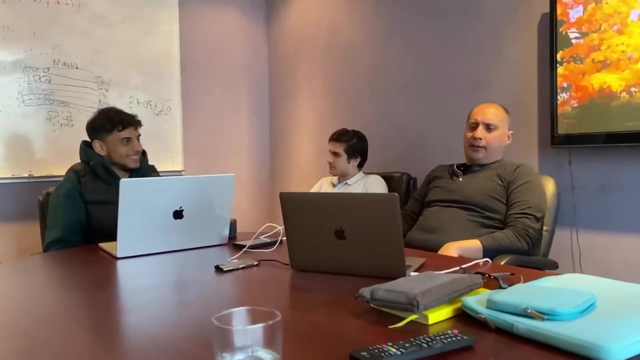 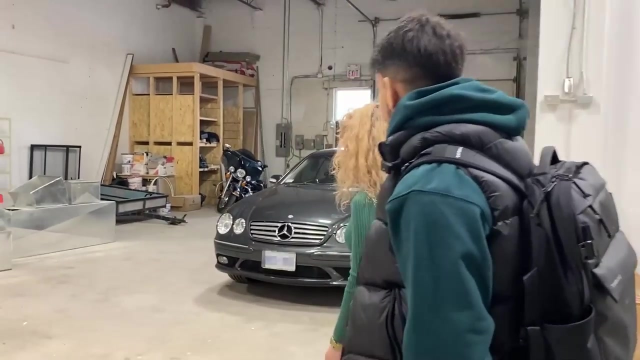 as well. yeah, we have a lot of space here too, so we have this space as well, a lot of desk space. hey, tamer, is that project done yet? oh shit, we're serious here. we use formulas for everything, even personal relationships. okay, so cool stuff to work with. whose car is that? this is the CEO's car he actually likes. 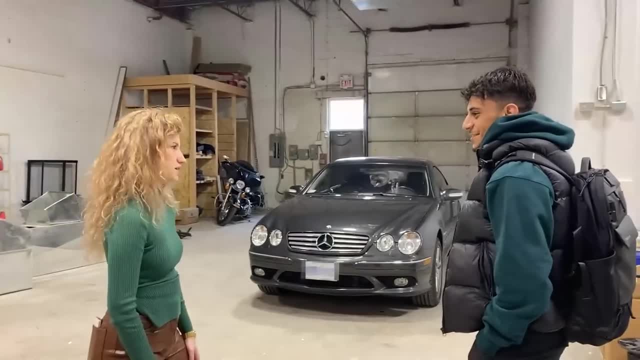 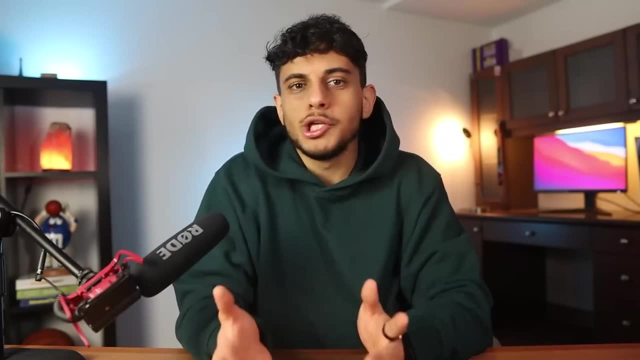 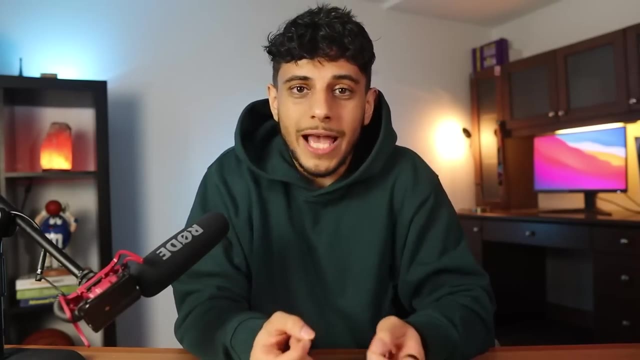 to like work on it. I hope this kid was entertaining and educational and give you a better understanding of what you can expect on your first day as an engineering intern. if you feel a bit unprepared for your first day and want a place where you can fill in your knowledge gap, then you should check out. 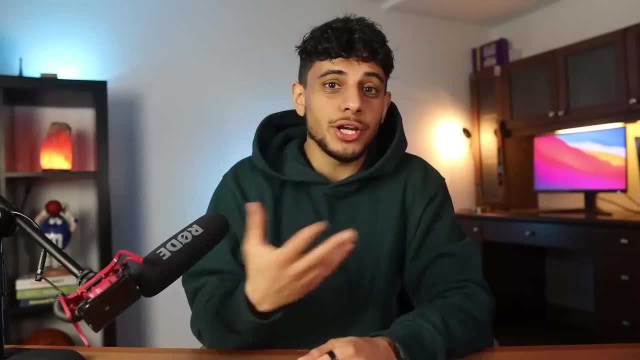 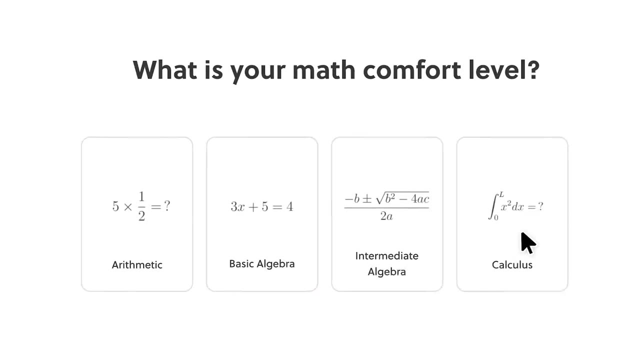 brilliant org or sponsoring this part of the video. as a mechanical engineer, my software skills are pretty weak. we didn't learn much about computer science fundamentals in my major, so brilliance hands-on computer science course has been super clutch in teaching me the basics, the advanced concepts to